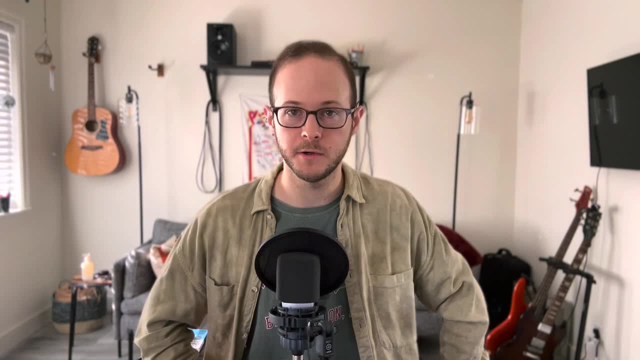 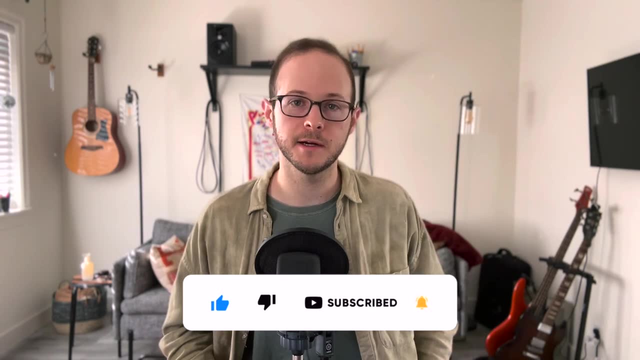 channel. I share all the lessons that I learned on my journey. So if you're new, kick back, enjoy the ride, Let's jump in, and if you really like this stuff, make sure to hit that subscribe button. I'm going to give a quick PSA here: Learning web development, learning software engineering. 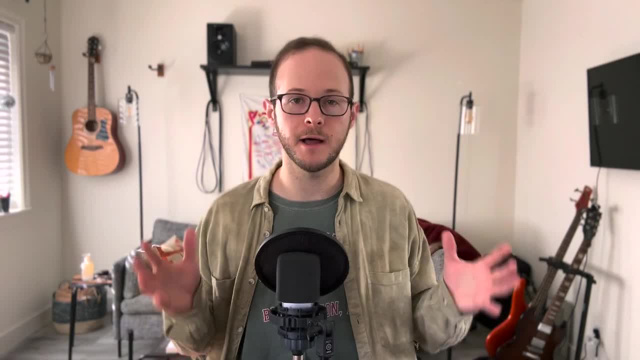 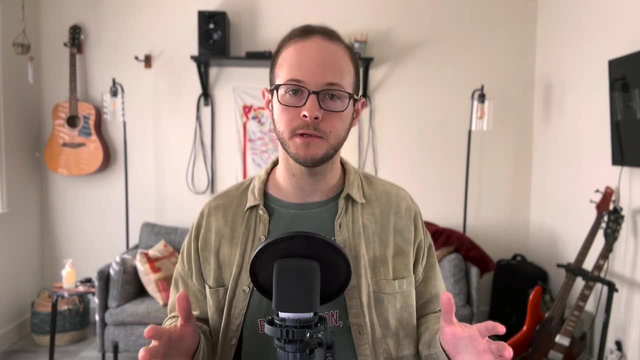 learning how to code does not take three months. You're going to see a lot of videos on YouTube telling you that you can become a Google software engineer in three months and make half a million dollars a year. That's not real. I wouldn't believe it. Coding is a lifelong learning process. It 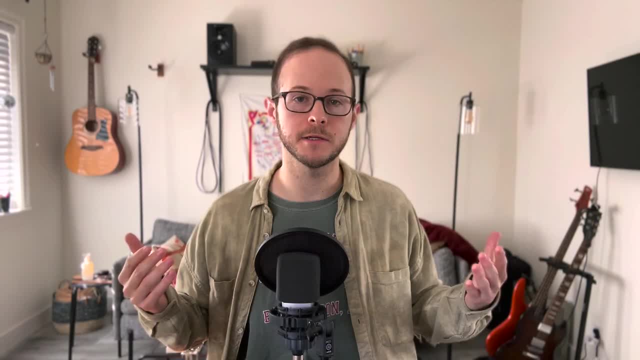 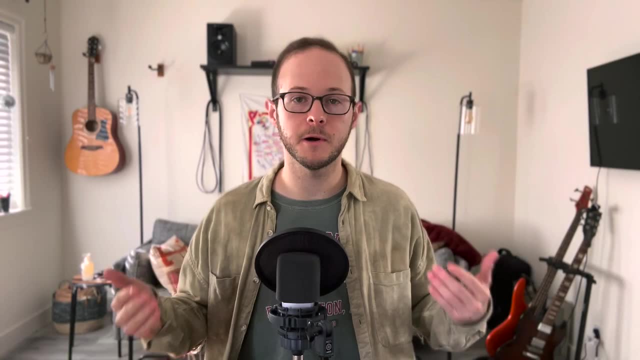 takes years to master. I'm only a few years in and I still consider myself to be an amateur. The second thing: don't do Harvard CS50. I'm not saying that it's a bad course, but a lot of people are going to steer you in the direction of taking 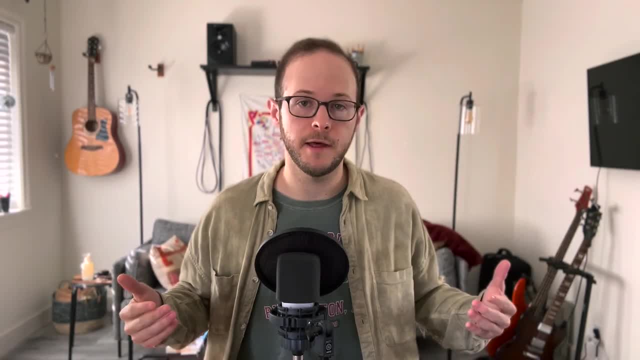 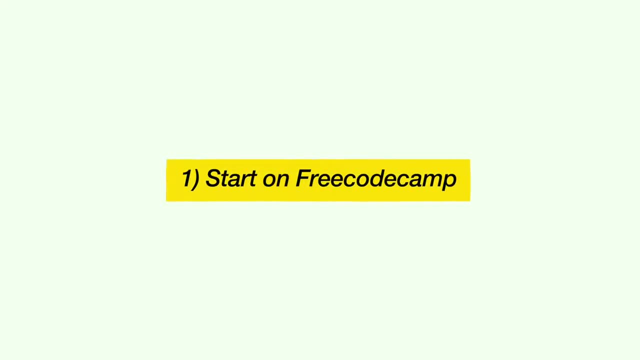 this type of course and personally I don't think that it's needed. I think that by taking a course like Harvard CS50, you're further just kicking the can down the road. If I were starting on day one, I would hop on Free Code Camp. I would start learning HTML and CSS in the basic web design. 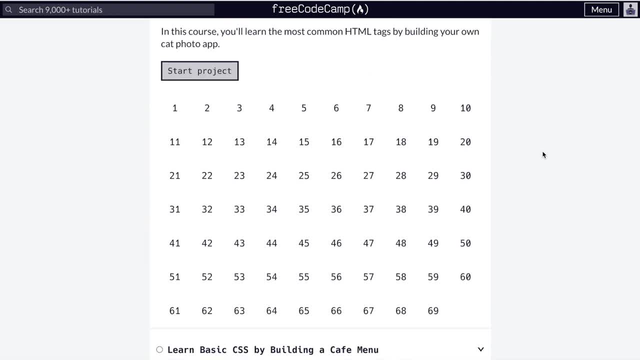 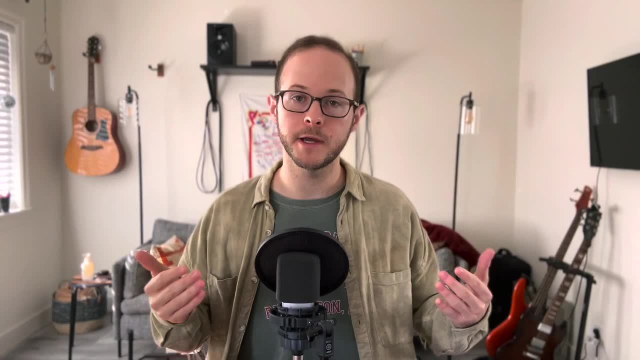 course that Free Code Camp offers. That's what I did. That's how I learned it. It only took me three months to learn. Mind you, I was really putting the hours in every day, so that's why I got through it in three to four weeks. So I think if you're committed, you can do it in less than a month. 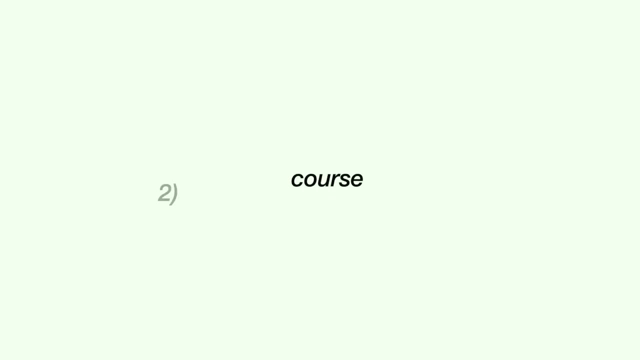 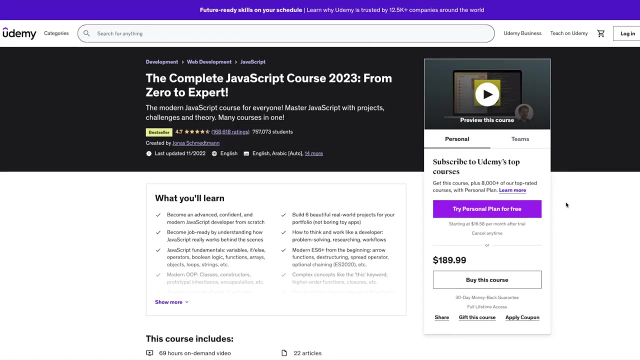 Once you've completed the web design track on Free Code Camp, I would go on to Udemy or something similar and take a JavaScript course and learn the basics. If I were doing it all over again, I wouldn't try to become a JavaScript master. Understand what a JavaScript function does. 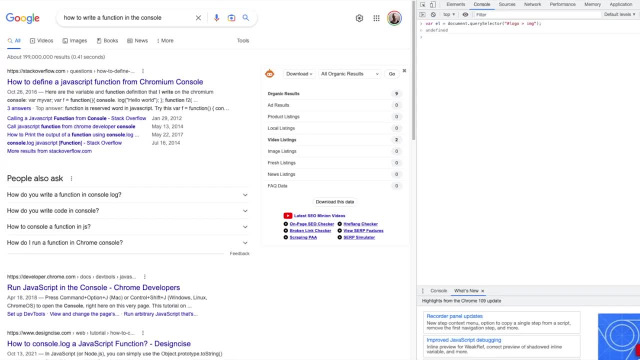 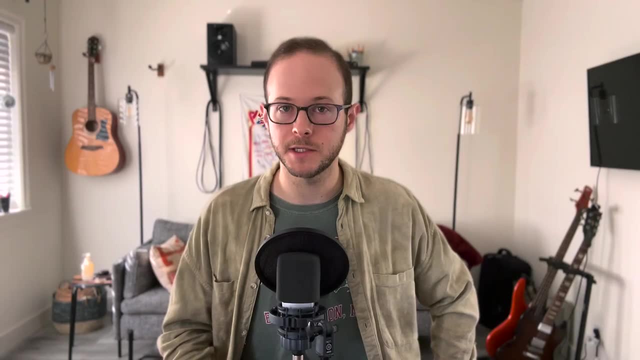 before you list that you're a web developer on your resume, Can you type out a function in the console? This is a super basic concept that you should know how to do. If you don't know how to do, this is basic JavaScript. Once you finish a basic JavaScript and web development course on. 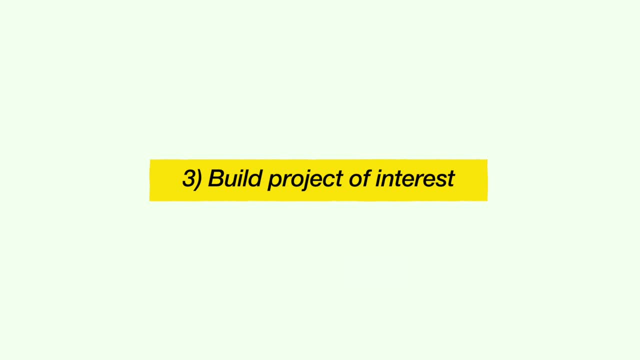 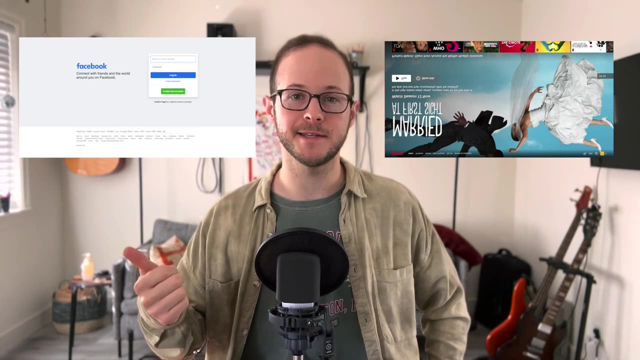 Udemy, I would build a project that you're interested in. Ask yourself what are your interests, What are your passions, What do you like? Don't build a Netflix clone. Everybody does that. Don't build a meta clone- Everybody does that. You should be original. Do something. 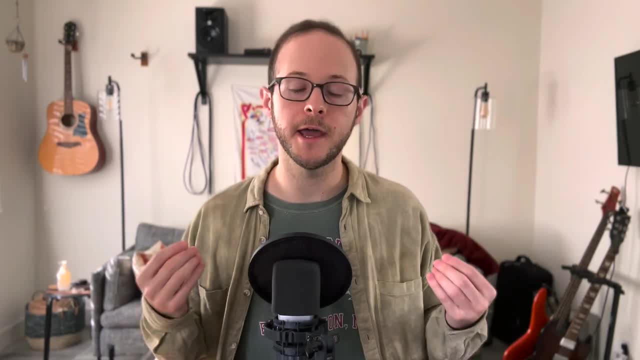 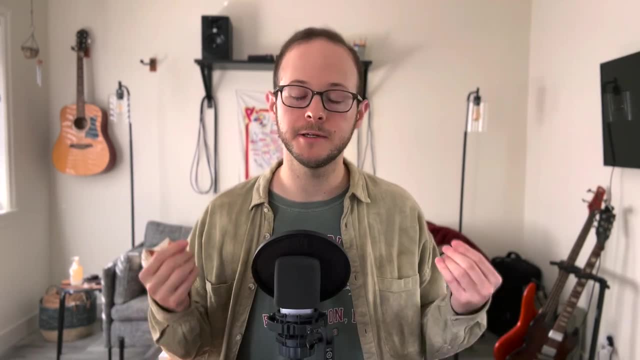 that is unique and something that you're passionate about, Not what everybody else wants you to do. An advantage of this approach is that when you're actually building the thing, you're more likely to learn what it is that you're working on, because you like the stuff that you're working on. It's 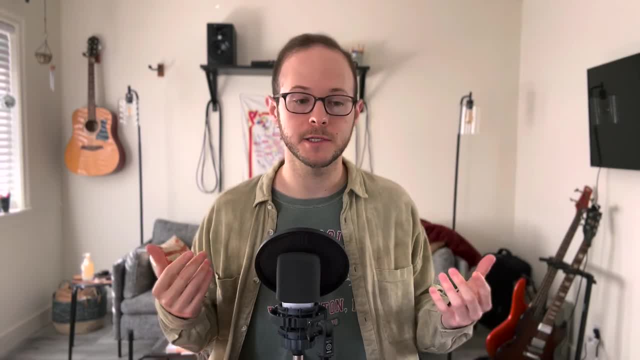 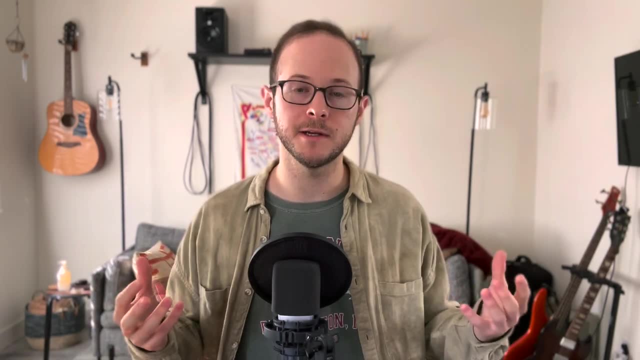 something that you're actually passionate about. So for me, I'm super interested in career development, so I built a job board in vanilla JavaScript and I really like doing that because I'm super interested in what it is that I was building. Make sure that you do it in the language stripped of. 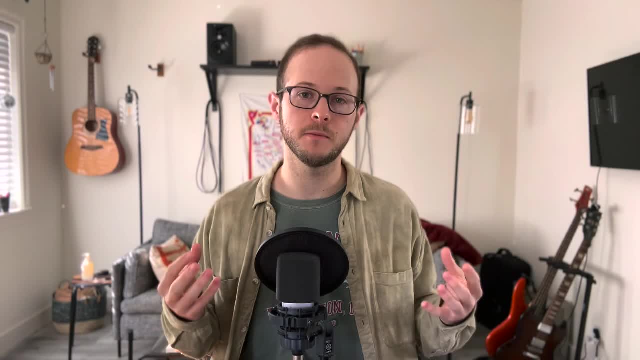 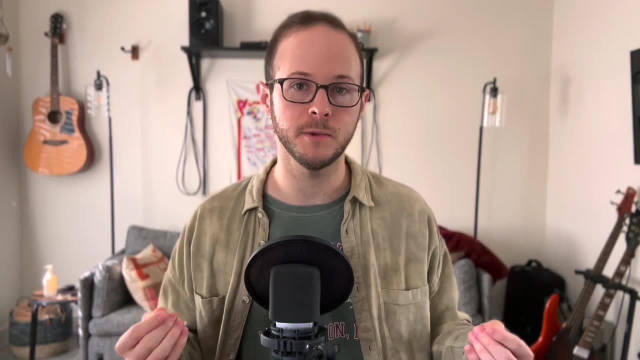 any frameworks. This is important because it reinforces the fundamental basics and understanding of the language of your choice. Like, you want to know the basics, like how to write a function, how to write a for loop in JavaScript. It's only until after you've built this project in the vanilla language of your choice that you 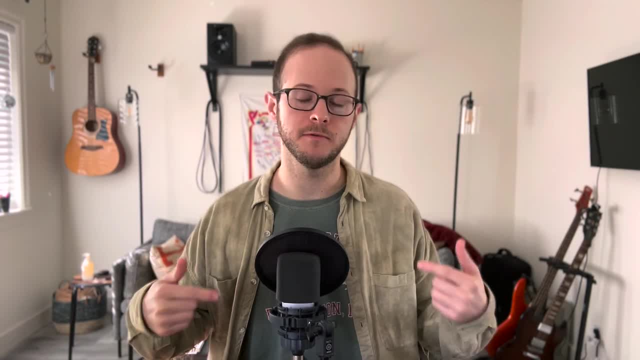 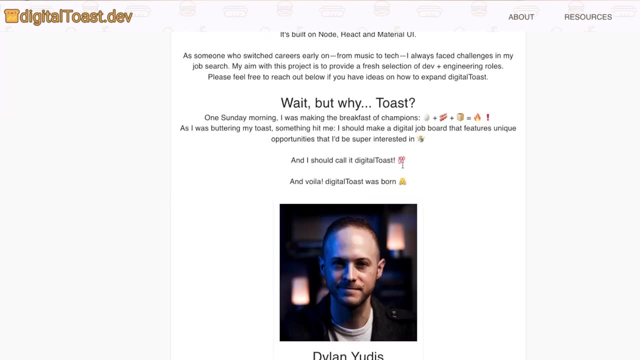 can build it in a framework. So after I was done building this project in vanilla JavaScript, I then decided to rebuild the project in the framework of my choice, which was React. I was able to better understand React as a result because, like, I really understood the basics of JavaScript. 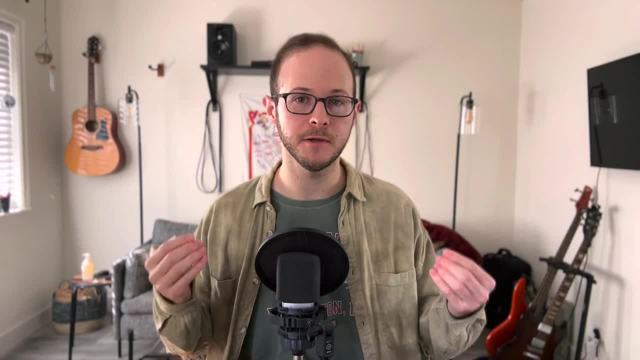 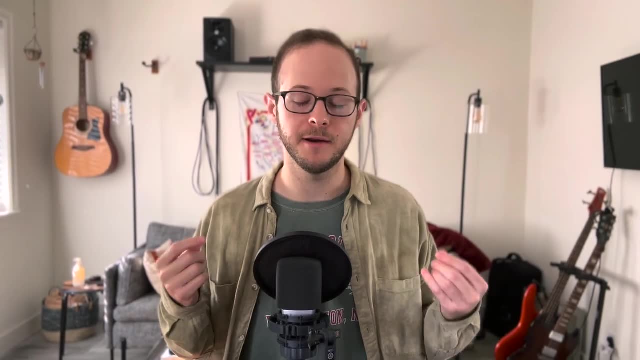 This is super important because a lot of people are going to tell you that you should immediately start building in the framework of your choice. Taking a quick pause here: this video is not about building a job. I've made a lot of other videos about that, which I'll link up here, but I wanted 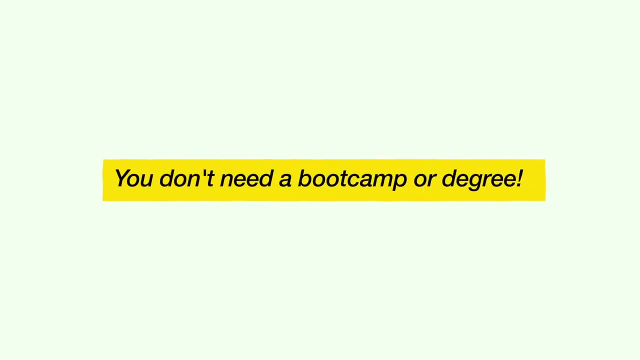 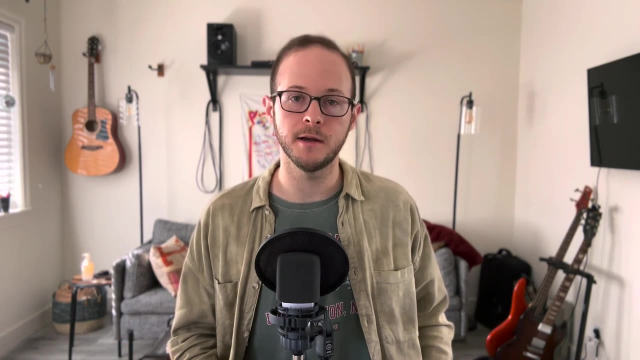 to say like: in my opinion, I don't think that you need to go to a boot camp and I don't think that you need to go back to school and get a CS degree. The main advantage of these two options is honestly just the structure that is provided, and you could also argue, probably the community too. But all the 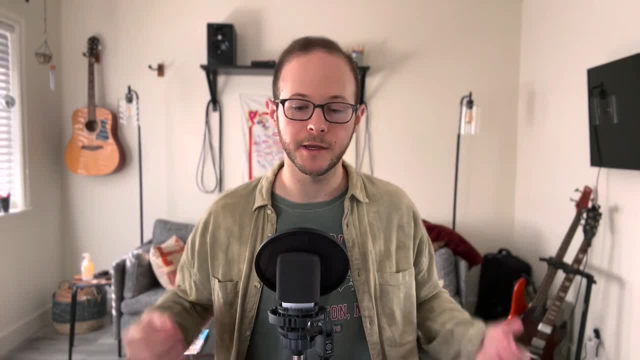 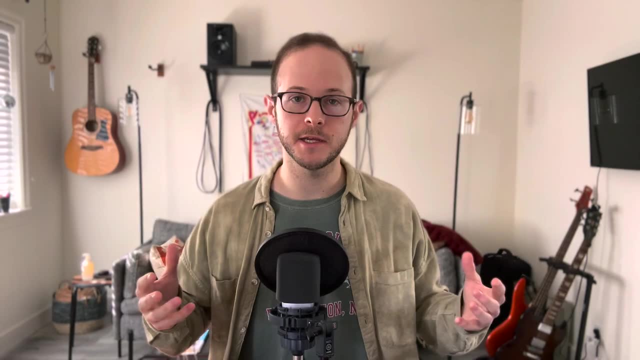 material that is offered. it's all free and cheap on the internet and like: if you want community, just go to a meetup. They're completely free and meetup organizers want as many people there as possible. Like: go to a meetup and ask people. I bet that you can figure it out at that meetup rather than 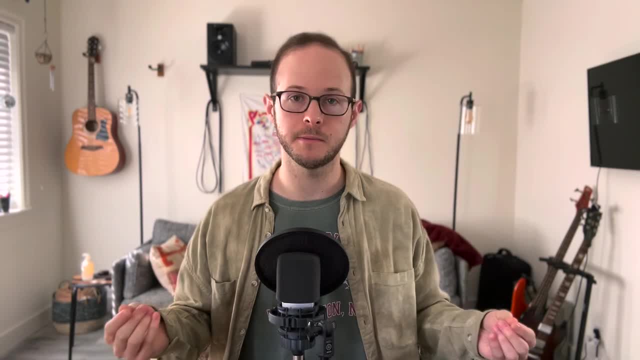 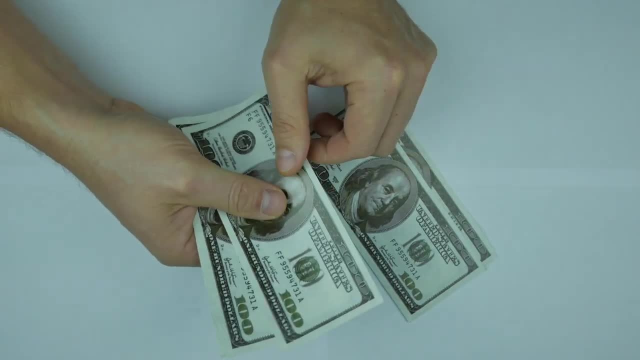 paying a bootcamp $17,000 for them to listen to your problems. for you A small rant: there's so many options like. there's so much out there and there's so many people trying to push you in the direction of paying them money so they can convince you that you can get a job in like. 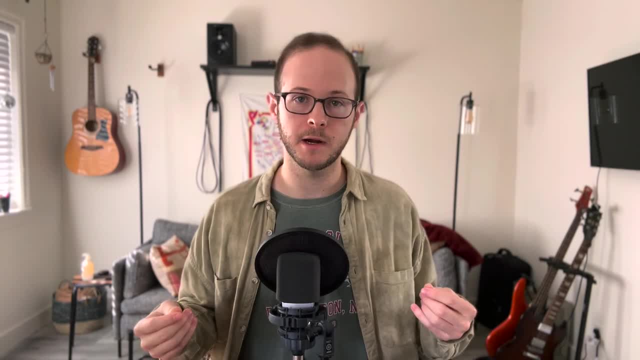 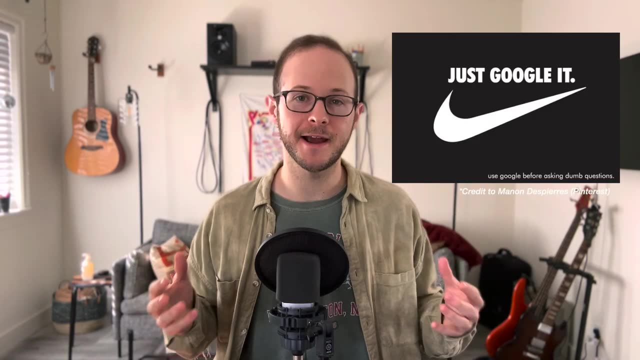 three months. Like you might be able to by doing one of these programs, but it's highly unlikely. like you have to put the work in. So my message is this: just google it. Like you're gonna have to google it and go on Stack Overflow whether you're in a bootcamp or doing a CS degree anyways. 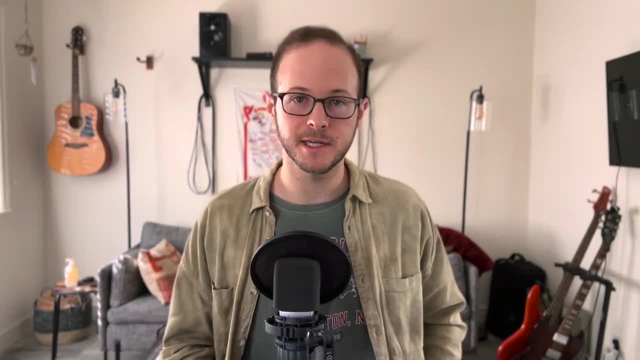 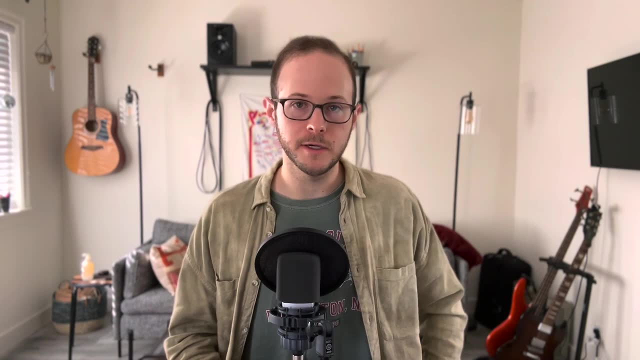 So, like you might as well just get really good at being resourceful yourself and, like I said, go to meetups for collaboration. Like if you have a bug or something, go to a meetup and I'm sure you guys are going to be able to figure it out. You can also use other resources like YouTube. YouTube is 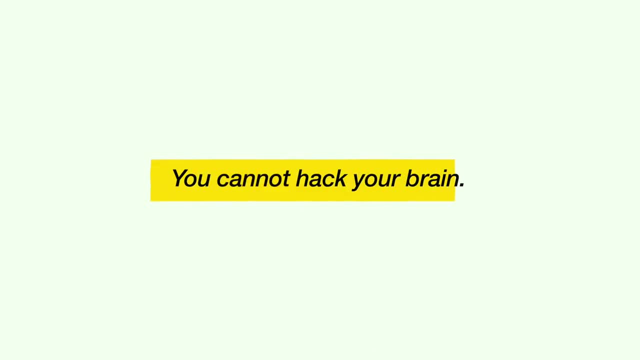 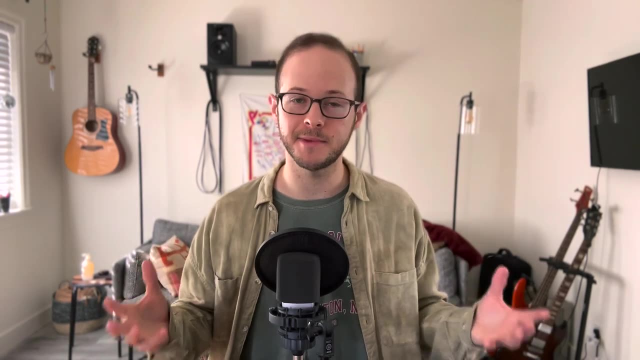 amazing. Stack Overflow is great too and, as I mentioned at the beginning of the video, like there's no hacking your brain, That's all a bunch of clickbait BS. Like you can't hack your brain to learn how to code. It's a brain, It's a muscle. I think it's a muscle Like you have to, just 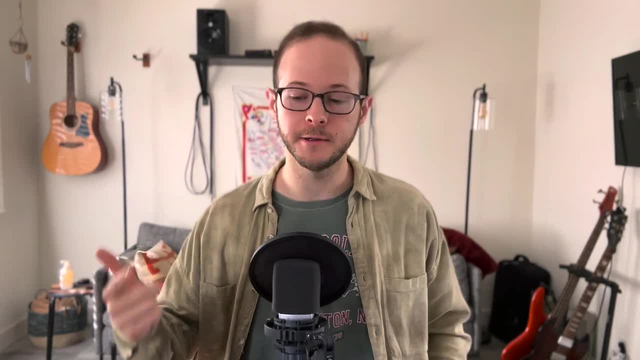 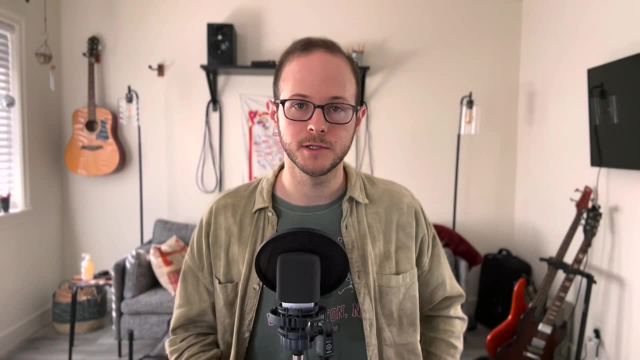 google everything You have to learn to be resourceful, Learn how to struggle and learn how to learn. It's not about the actual coding language or web development technology itself. It's learning how to learn the actual tech. So, in summary, if I were just starting out, I would hop on. 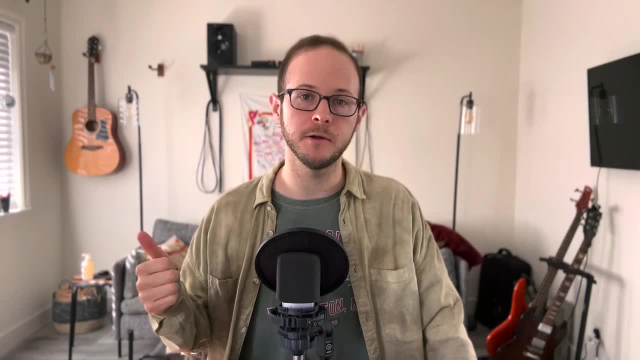 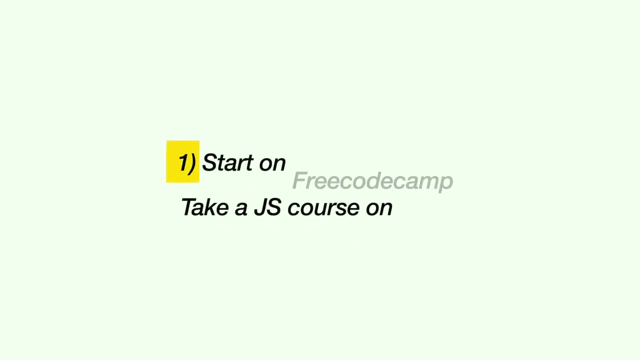 Free Code Camp and do the web design course. It's totally free and you'll learn HTML and CSS. If you put in the work every single day, you'll probably be able to get through it in three to four weeks. Then I would hop on Udemy and take a JavaScript focused course or something that's a little more. 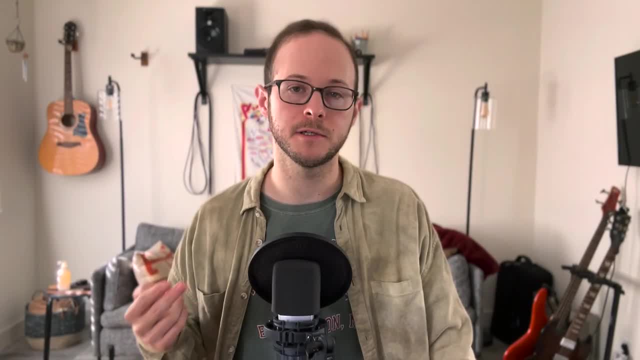 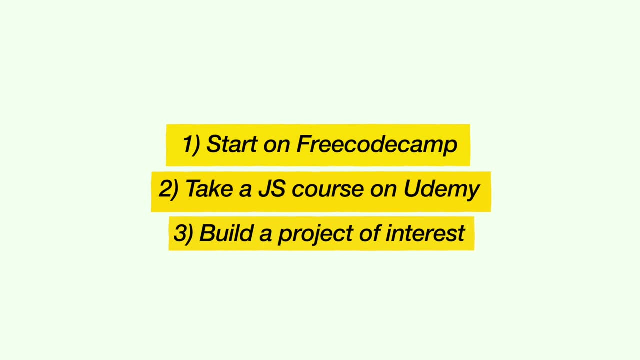 comprehensive in web development. I'll link a couple of the example courses in the description and focus on just getting good at the basics of vanilla JavaScript and then take all those skills that you just learned from the last couple of courses and build a project based on something that you're passionate about. Don't build a Netflix clone. Everybody does. 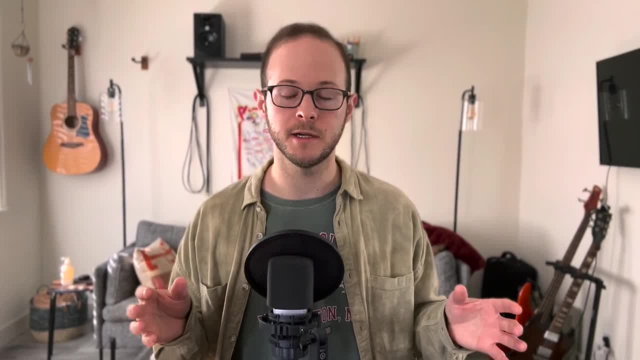 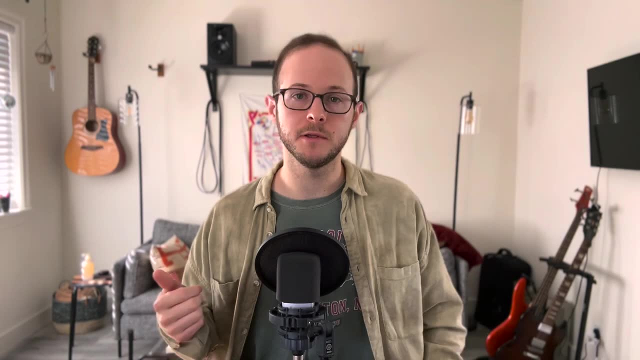 that You want to be original and also the advantage of doing something that you're interested in is that you're more likely to keep doing it because you're interested in doing it. Then, when you're done building that project in vanilla JavaScript, you can rebuild it in the. 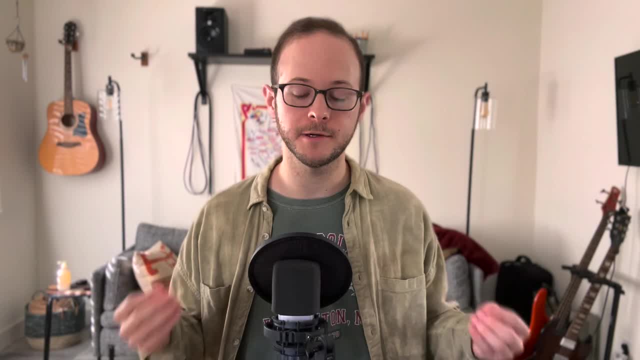 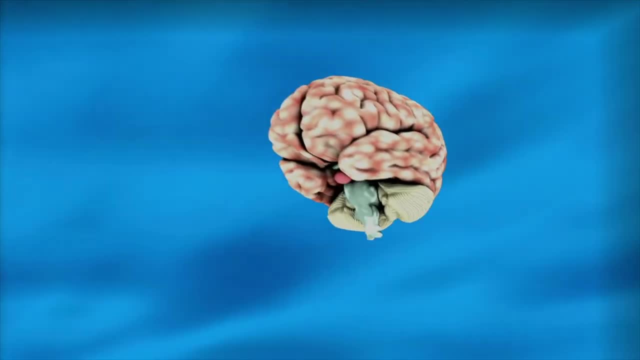 framework of your choice. And, lastly, you have to learn how to struggle. You have to learn how to learn Go and Google it Like there's no brain hacks this stuff. You can't hack your brain and become more productive and learn how to code. This is stuff that people try to sell you on. 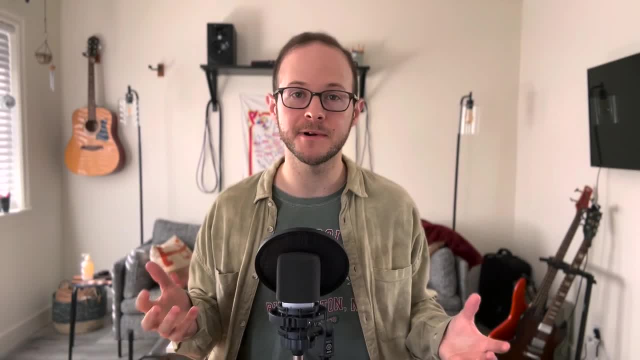 the internet Like it's a brain. Come on, you can't hack it, It's not a computer. Learn how to struggle and how to gird through problems the real way, The way that everybody else does it, So don't buy into. 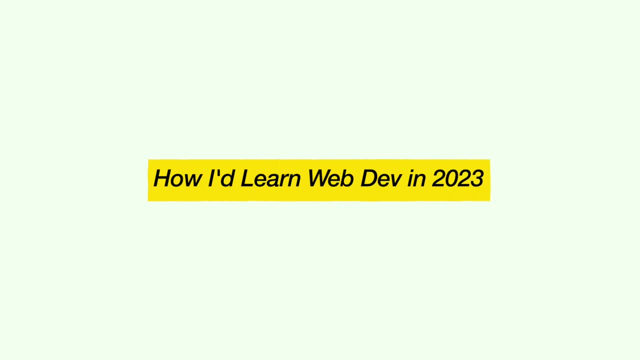 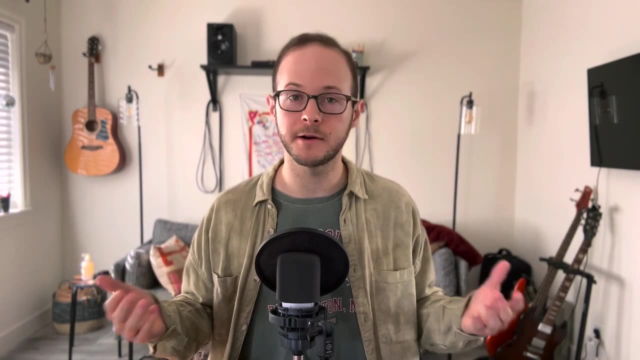 the BS. Anyways, that is how I would learn how to do web development in 2023 if I were just starting out Again. this is my bold take. This is what I see on YouTube and what I disagree and agree with, So if you like this content,